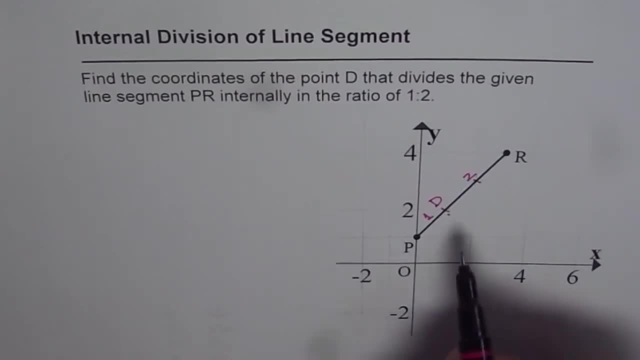 So that is how we can easily get our answer. and we know coordinates of point D are 1,, 2. Done. So if a coordinate plane is given to us, is that right? That's simple. So the concept is: take a line, divide it into number of parts, which is sum of those ratios, and then easily we can pick up the point. 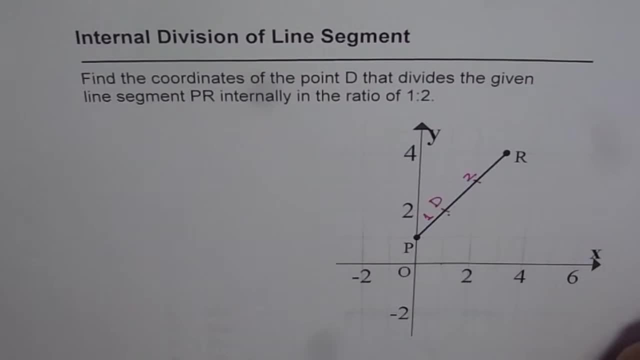 Now how to do this as an exercise for vectors. That is what we are going to explore Now. for vectors, as you know, points- We can treat these points as position vectors. So what we will do is we'll refer to origin and let's consider O as an external point, and from O we will draw the vectors OP and OR. 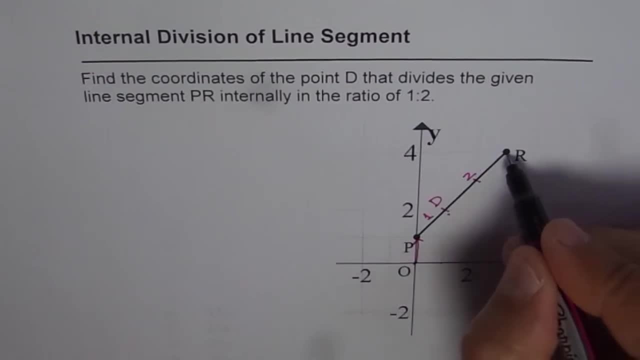 So we have these vectors now which are OP and OR. right, Let me draw it with the dotted line first. Okay, so good enough, So let me just join it. So we have OP and OR, And what we need, What we need to find, actually, is somewhere in between: a point D which divides the line PR in the ratio of 1 is to 2.. 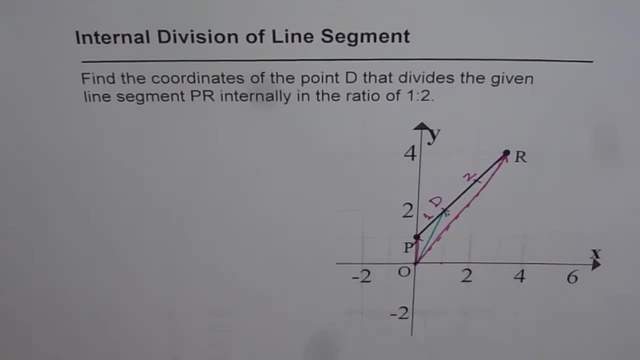 Now the question is how to find that point. So now we'll use the concept of vectors to find the point D. We already know our answer right. The answer is 1, 2.. Let's see how do we get it. 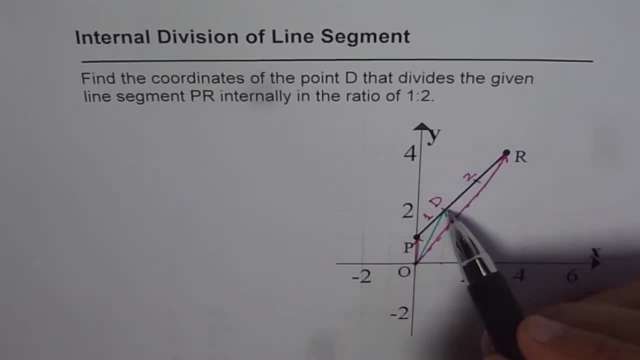 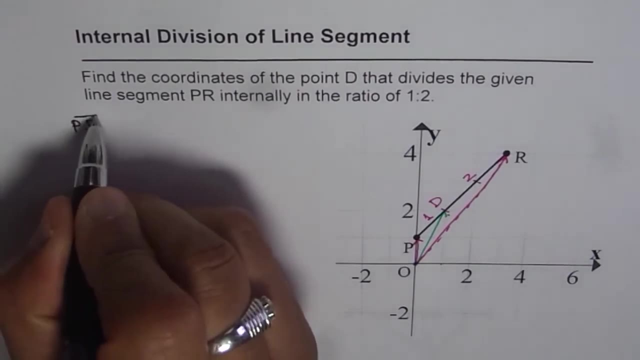 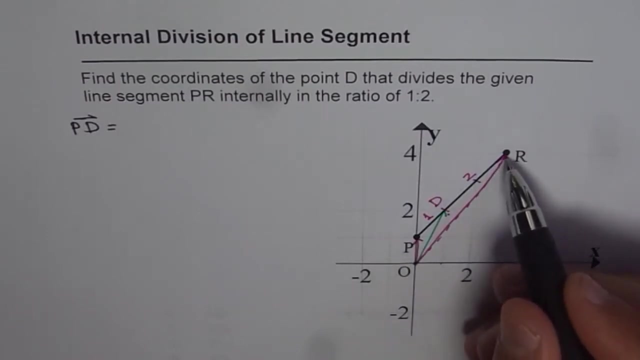 So now We can say that D Let's say what is PD. PD can be written as It's a scalar multiple of PR, correct? And if PR has a length of 1 plus 2, which is 3, then PD is 1, right? So it's one-third of PR. So I can write this as one-third of PR. 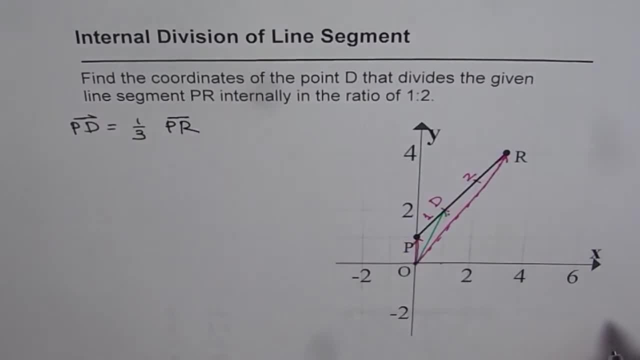 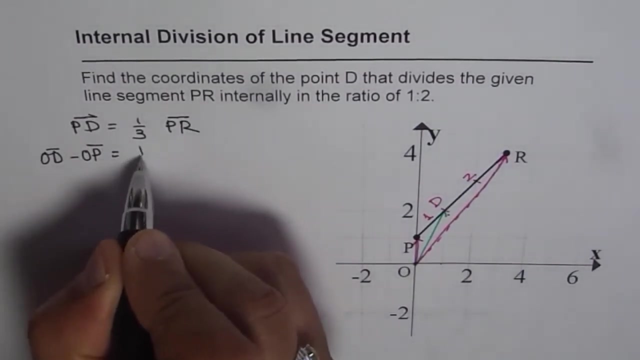 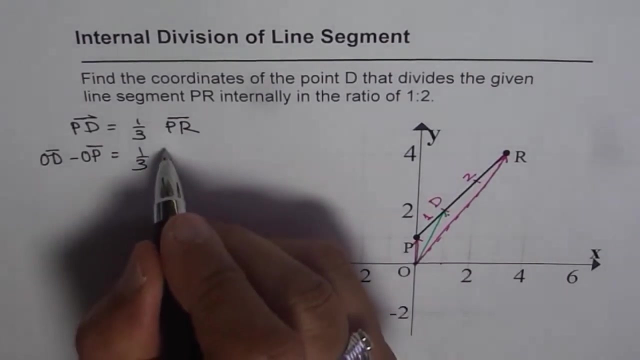 Right, So that's how we get PD. Now, PD could also be written in terms of OD. We can say PD is OD minus OP, So we can write this as OD minus OP. It's one-third of PR, and PR can be written as OR minus OP. 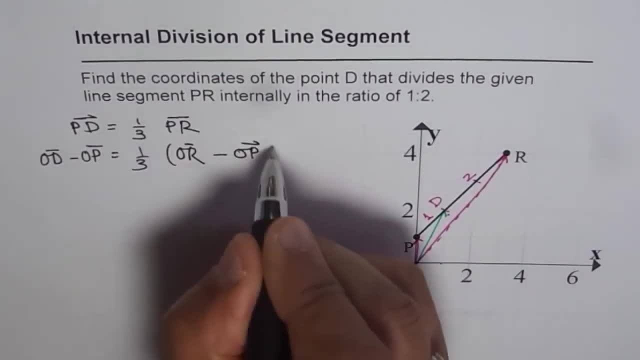 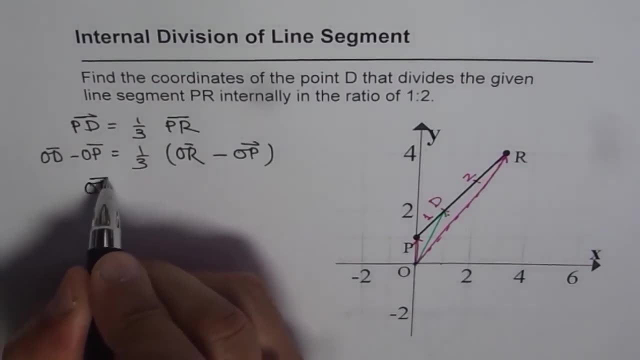 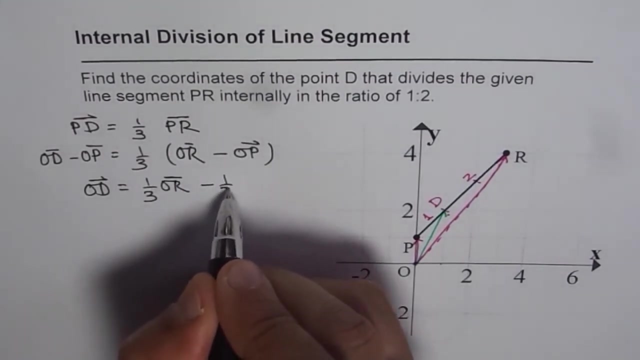 OR minus OP, Correct. And here we can find the position vector OD. So OD is equal to. Let's expand this: We have one-third of OR minus one-third of OP And we bring it here. We get plus OP, right. 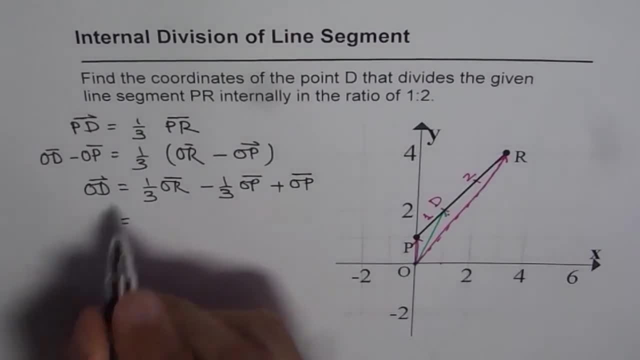 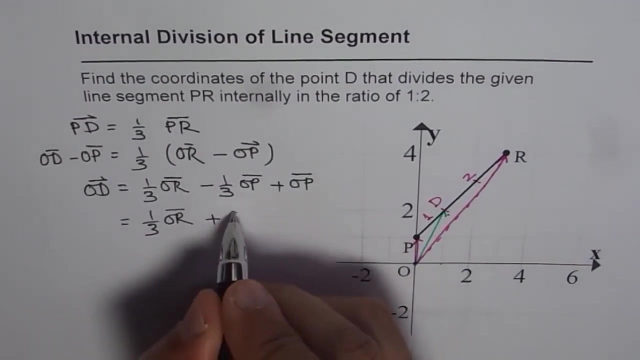 So we get OD the position vector That will give us the coordinates also, right. So let's combine these two terms. We get one-third of OR minus one-third. One-third from plus one gives us two-thirds, right, So it is two-thirds of OP. 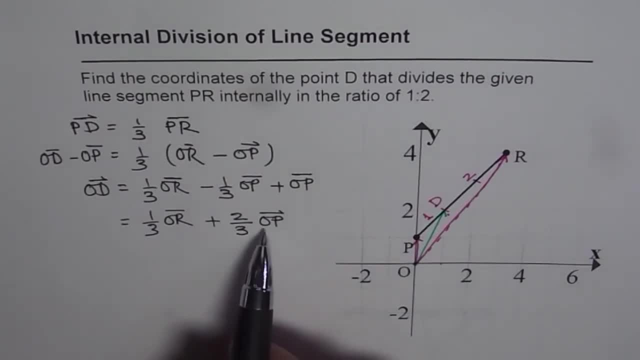 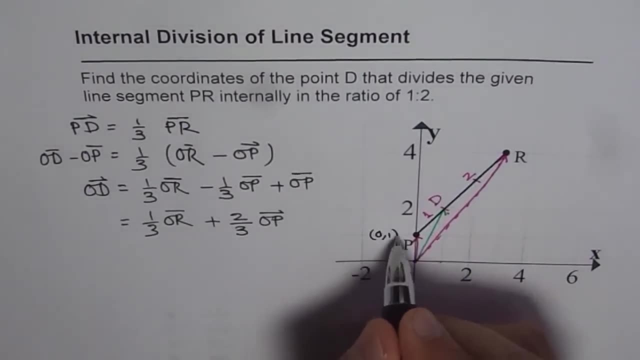 That's what OD is. Now we know what is OR and we know what is OP. OP is 0, 1,, right, So OP is 0, 1, and OR is 3, 4 for us in this given scenario. 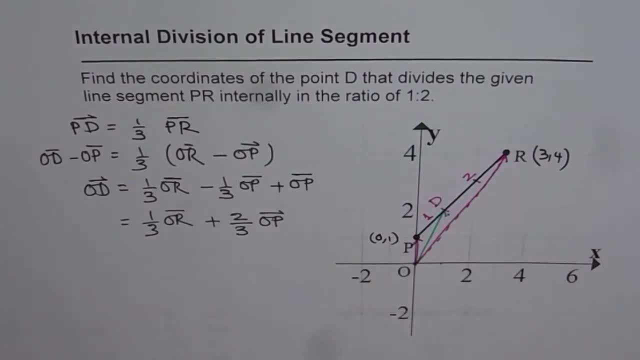 So we'll utilize these points and find the coordinates of point D, So we can write this as 1 over 3, OR is 3, 4, plus 2 over 3 of 0, 1.. And that gives us one-third of 3. is 1, 4 over 3, plus. I mean 0, 2 over 3, right. 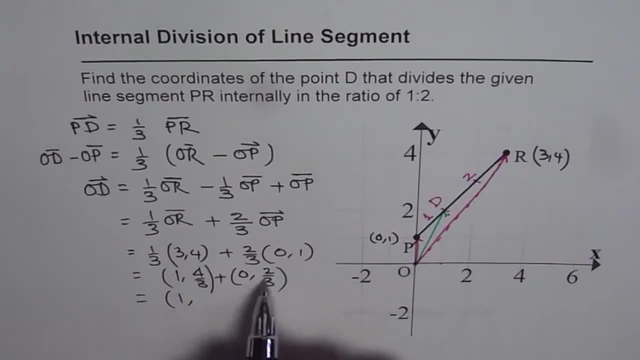 And that is 1,, and 4 over 3 plus 2 over 3 is 6 over 3,, which is indeed 2.. So vector OD is 1,, 2. And that means point D should be what. So from here it's very clear. that implies that point D basically is 1,, 2, right. 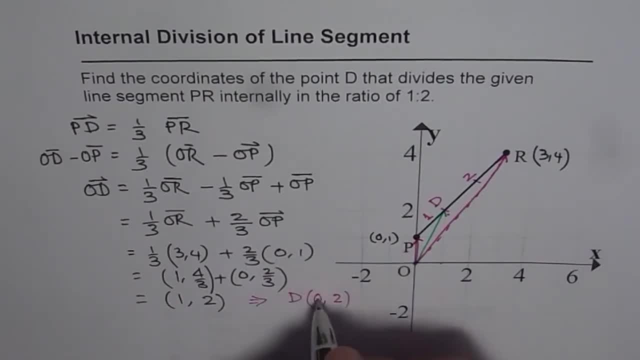 From origin. oh sorry, I wrote is 1,, 2, right. So that is our answer. So we can now write down our answer as The point D that divides the given segment PR in the ratio of 1 is to 2 is 1,, 2, right. 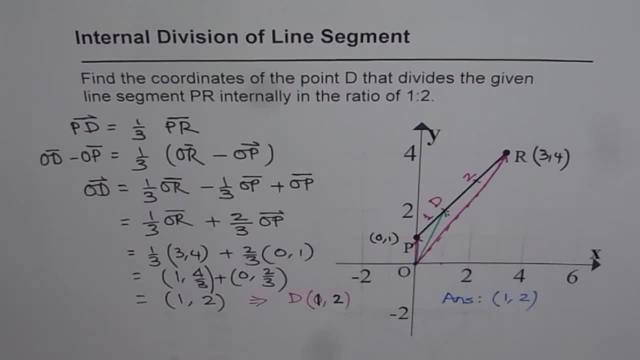 And that's the vector way of doing it right Now. this is such a beautiful method that it could be adopted whether you have a 2D or R3. It doesn't matter, right? So you could adopt this method in solving any problem.